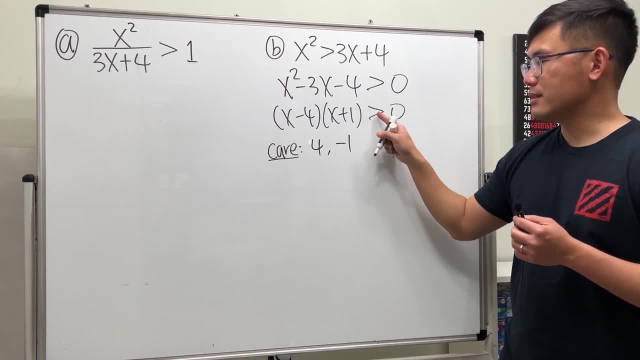 So two numbers that we care, But we don't want to include them because it's greater than I know. it sounds kind of bad. huh, We care about these two numbers but we don't want to include them. That's just life. 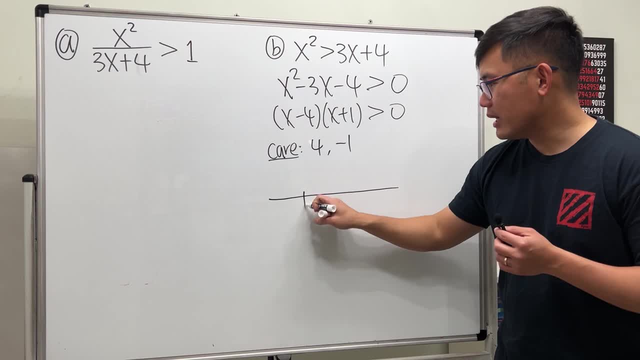 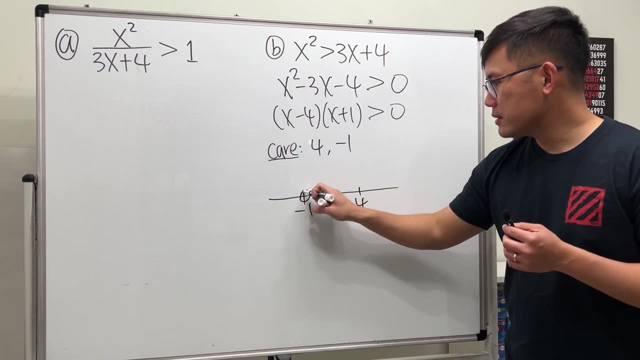 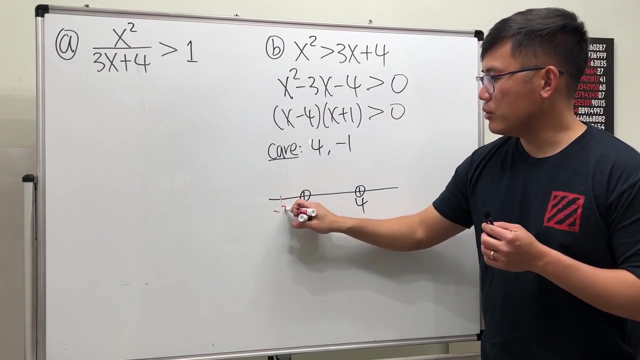 Anyway, here, draw the number line, Put a negative 1 to the left because it's smaller, And then the 4 right here. Alright, open circle. open circle because we are not including this and that. Huh, Now pick a number less than negative 1,, let's say negative 2.. 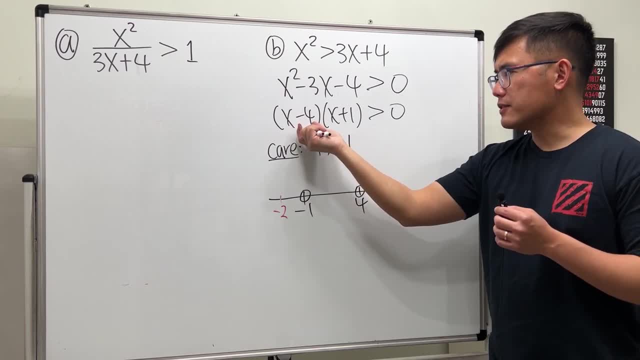 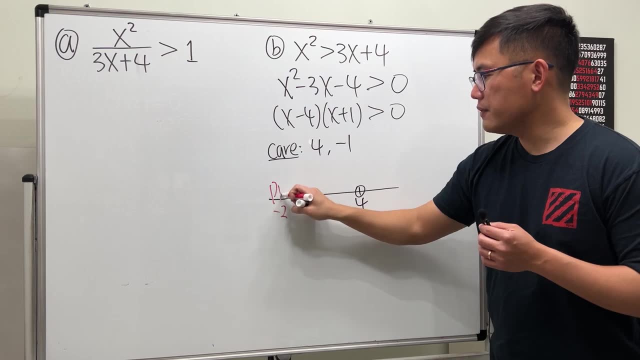 Put it here: negative 2 minus 4 is negative 6, it's negative. Put it here: it's negative. Negative times negative. we get positive. Then we do the same thing. Pick a number between negative 1 and 4, let's say 0.. 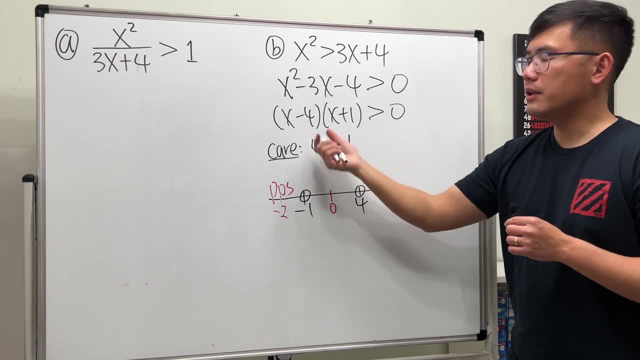 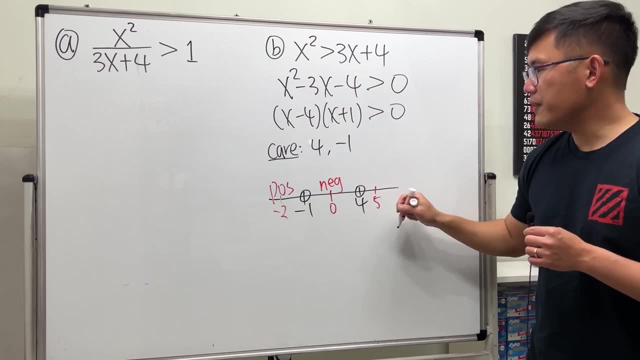 Put it here: we get negative. Put it here: we get positive. Negative times: positive is negative. Pick a number bigger than 4.. Let's say 5.. Well, this is positive and this will also give us positive. Together, it's positive. 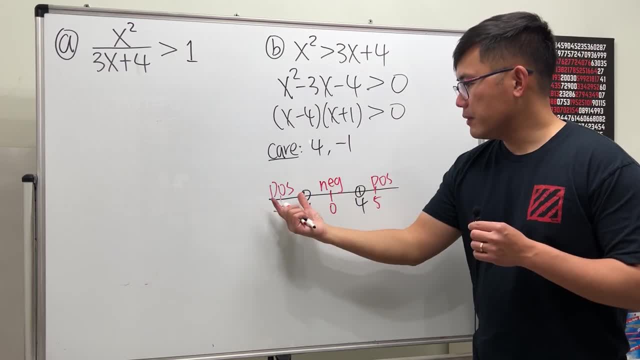 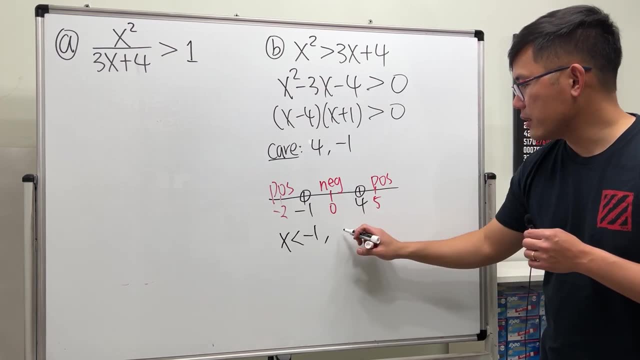 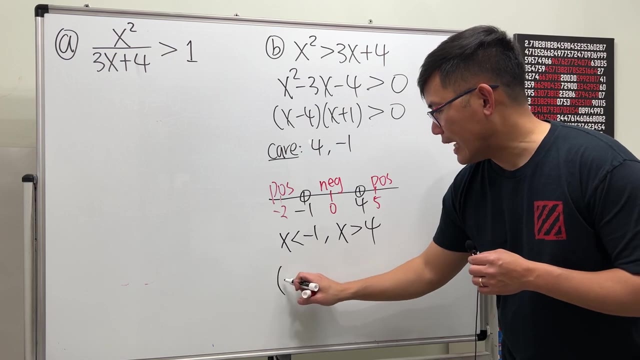 As you can see, we care about the positive parts, which is this and that? So the answer for this is x is less than negative 1, or the other one is x is greater than 4.. So two different intervals. And now let's write the interval notation which we have: negative infinity to negative 1.. 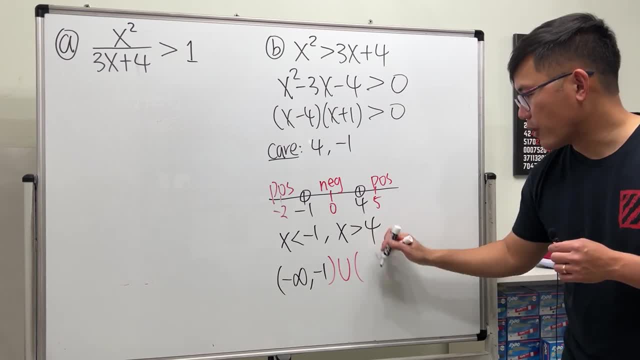 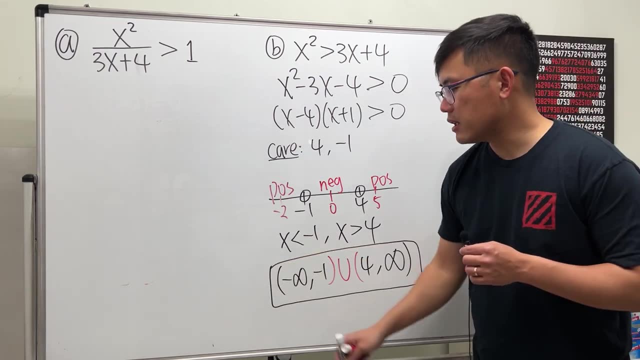 Do not include the negative 1.. So negative 1, union, we go from 4 to infinity. So it depends on how you would like to present the answer. Usually it's in the interval notation once we are in the precalculus class. 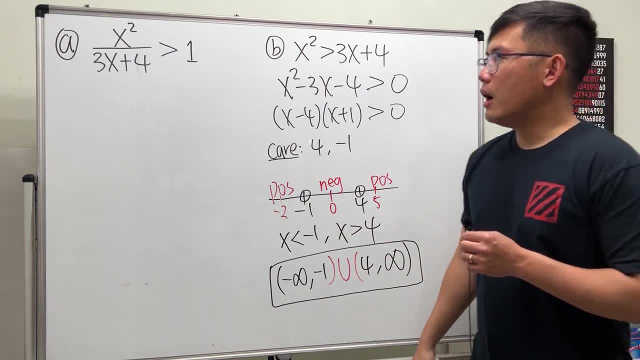 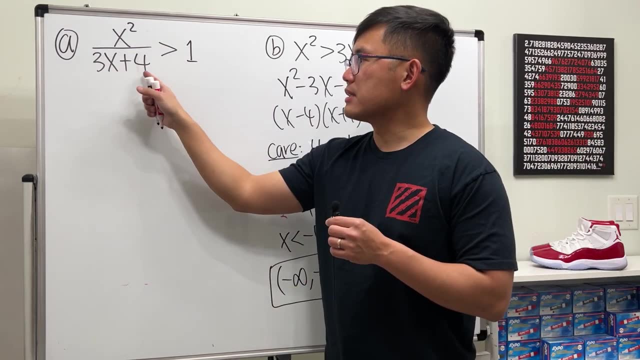 But don't forget these notations as well. All right, now, how are we supposed to deal with this? The problem is, when we have the 3x plus 4 on the bottom, you have that extra cut point, right, Because? 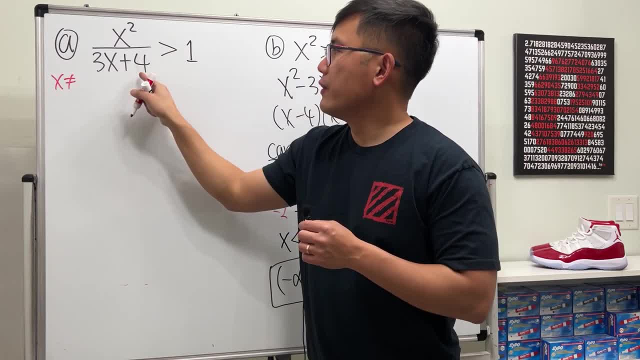 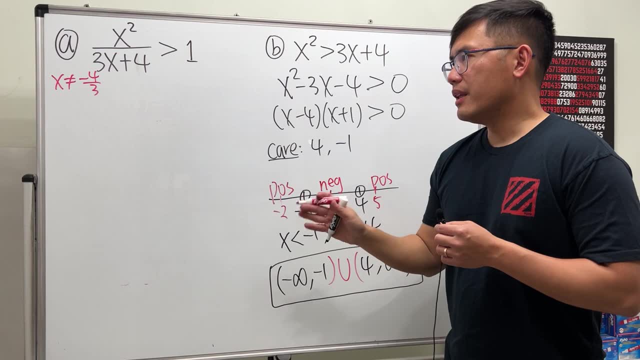 Here x cannot be equal to negative 4 over 3, because that will make the bottom equal to 0. So too bad. That is the trouble number 2.. But earlier, when we have nothing on the bottom, don't worry about it, right. 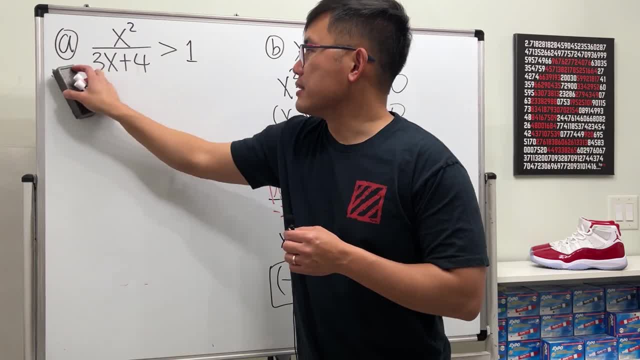 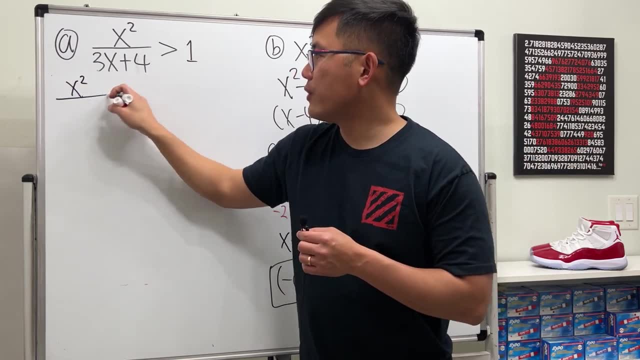 So keep this in mind. Now let me show you guys a safe way to do this. Firstly, put a 1 to the other side. We are going to get x squared over, 3x squared, x plus 4. And then that will be minus 1.. 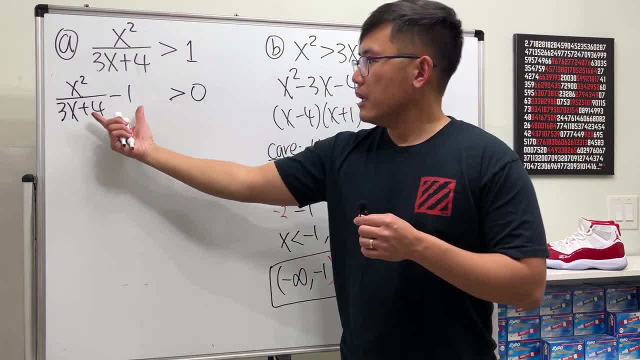 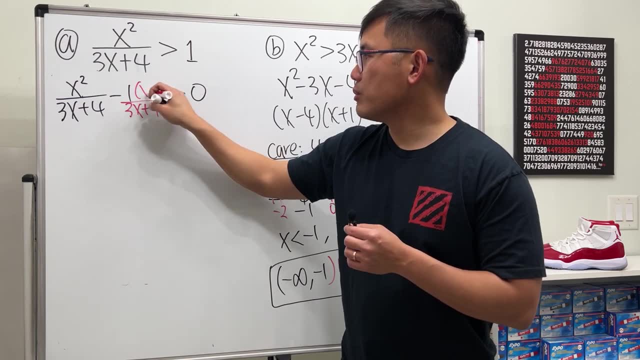 And that will be greater than 0.. Next, we are going to combine the fractions. Here we need a common denominator, which is 3x plus 4.. And let's also multiply that on the top as well: 3x plus 4.. 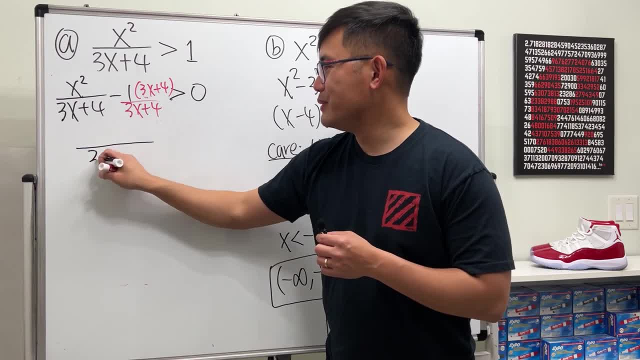 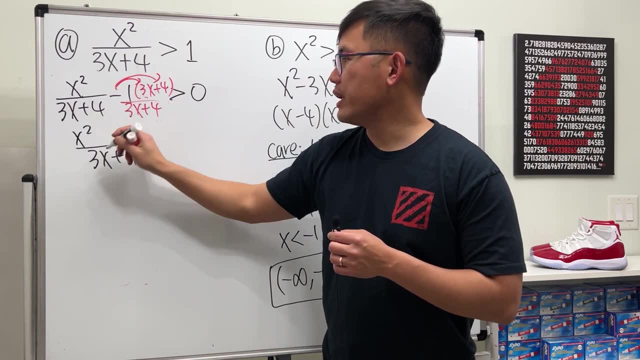 So altogether we can put them together. Altogether we have 3x plus 4 on the bottom. On the top this is x squared And then distribute the negative 1. We get Negative. 3x minus 4 is greater than 0.. 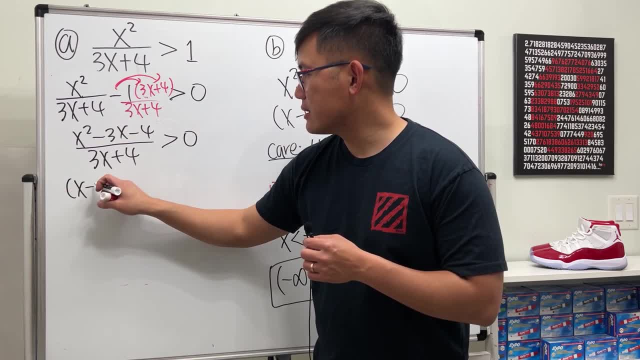 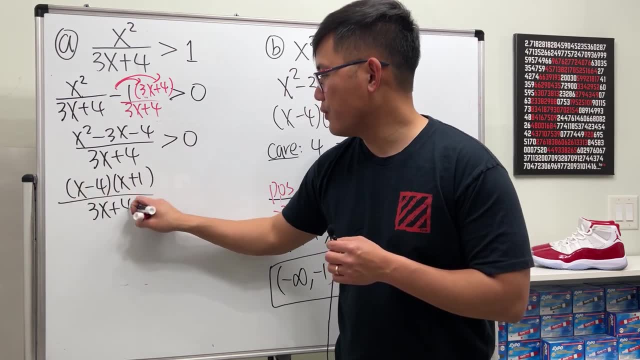 As you can see, on the top we get x minus 4 times x plus 1. Over the bottom we have 3x plus 4. And that's greater than 0. Here we have 3 factors to consider. 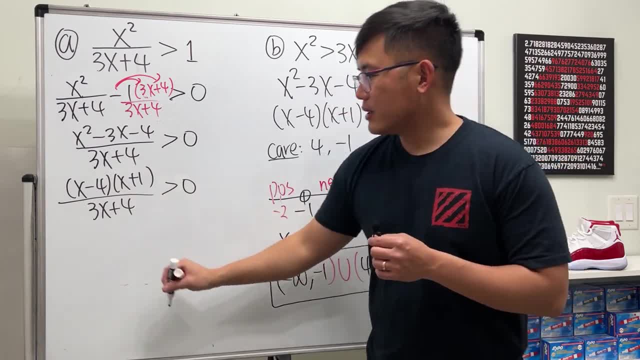 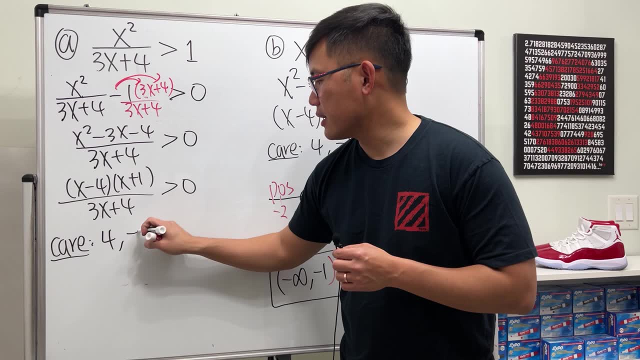 This, this and that. Alright, so here are the numbers that we care. From this we care about 4.. From here, we care about negative 1.. And from here again, you just put it to be 0.. 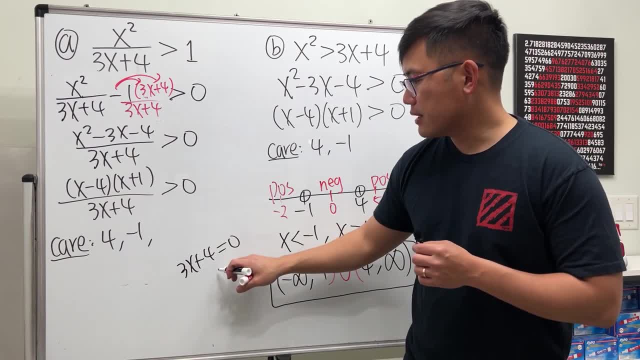 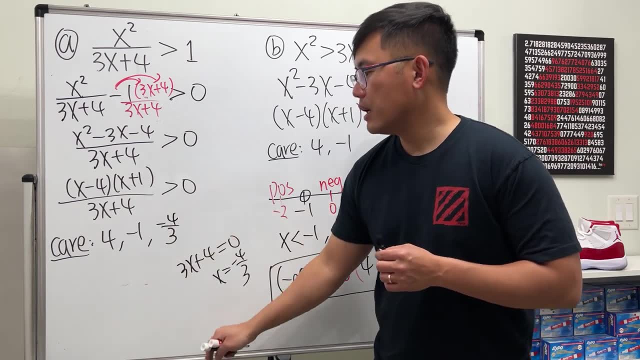 That's how you find out the numbers you care. Move the 4 to the other side. Divide it by 3.. x is equal to negative 4 over 3.. So we also care about negative 4 over 3.. We care about all this, but we do not want to include that. 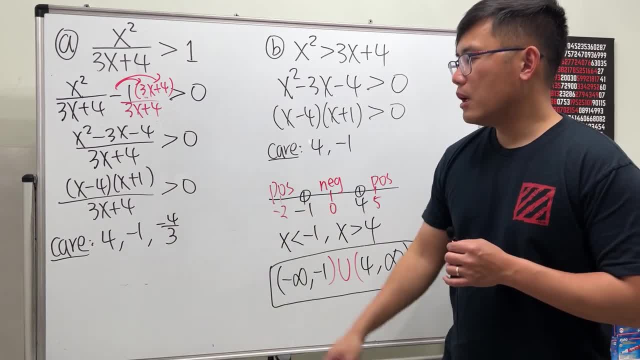 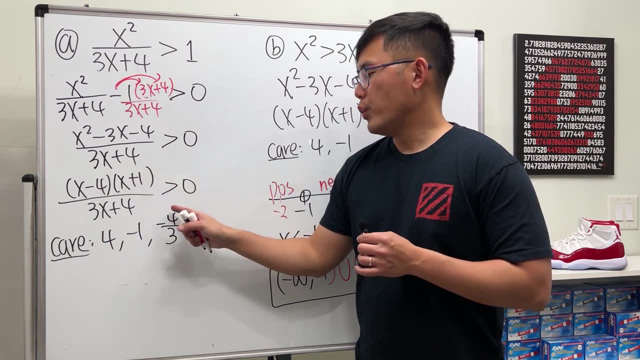 because it's just greater than There's no equal sign. If there was an equal sign, then we are going to include the 4.. We are going to include the negative 1. But we will still not include the negative 4 over 3. 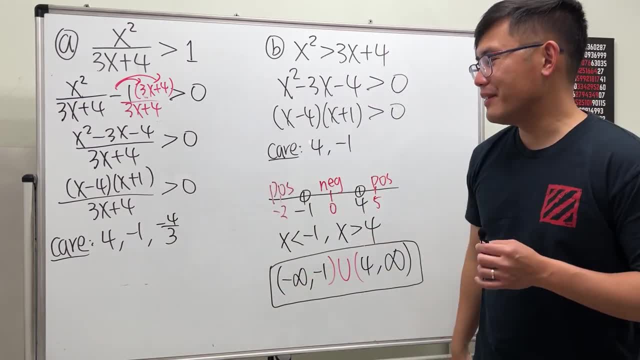 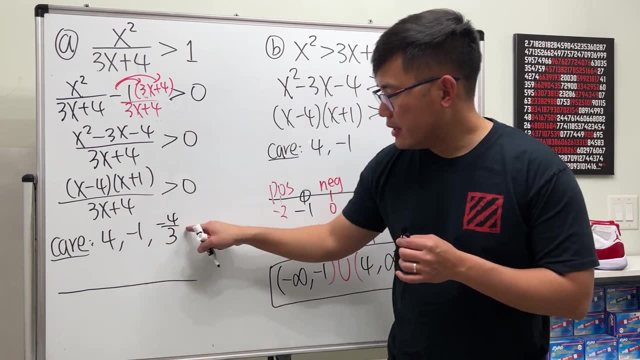 because that's on the bottom. That's just the reality when you have the expression on the bottom. Okay, here we go From the smallest to the biggest. This right here is the smallest, which is negative 4 over 3.. Next we have negative 1.. 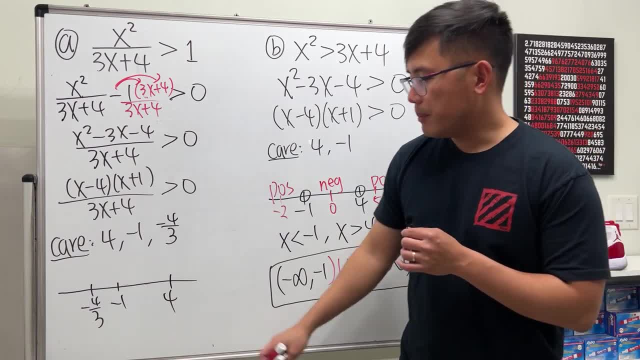 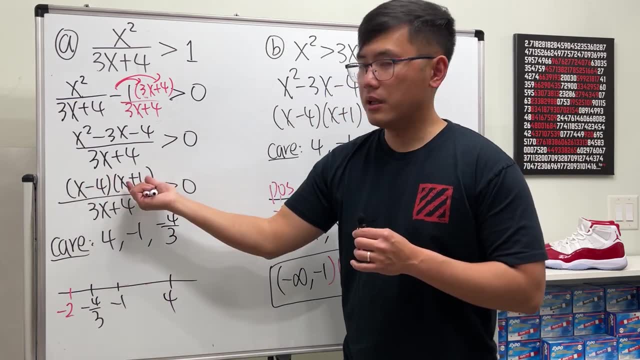 Next we have 4.. Let's put it down right here. Okay, pick a number that's the negative: 4 over 3.. Let's say negative: 2.. Put it here: Negative. Put it here: Negative. Put it here. 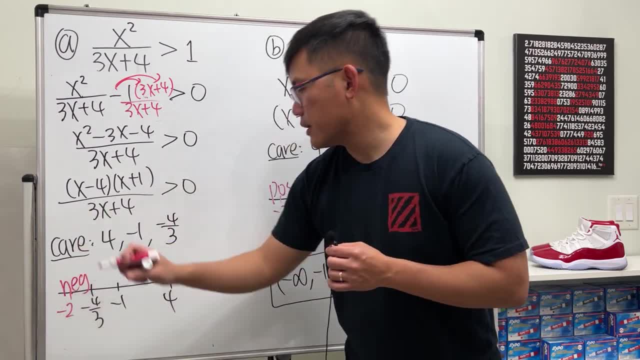 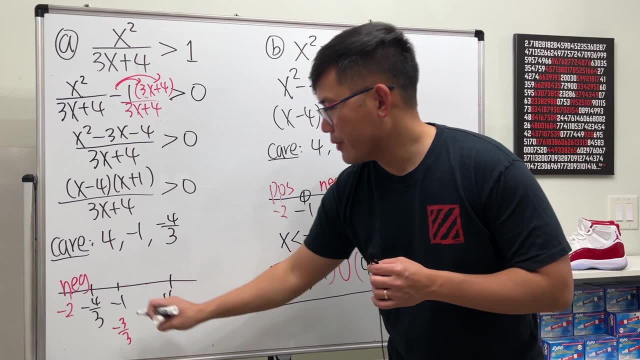 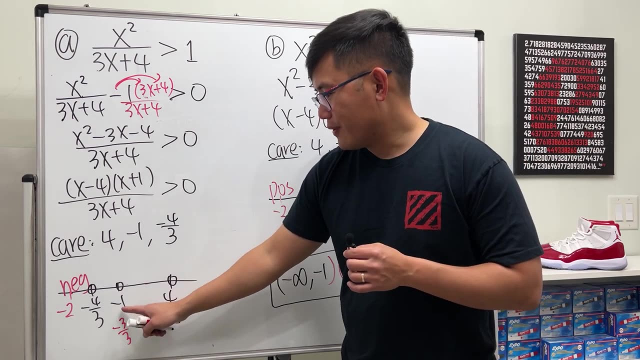 Negative, Altogether negative. Next, this right here is a little bit trickier. This is like negative 3 over 3 for the negative 1.. Oh, by the way, open circles for all of this, To pick a number in between of this and that. 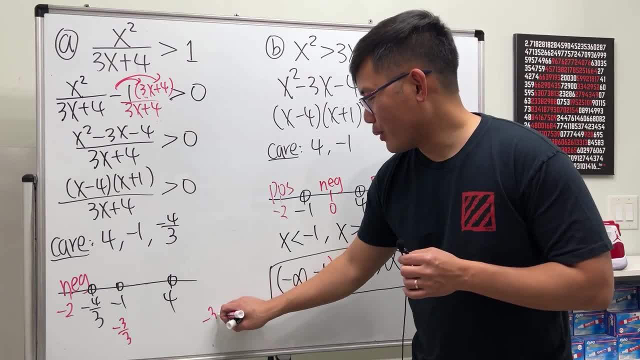 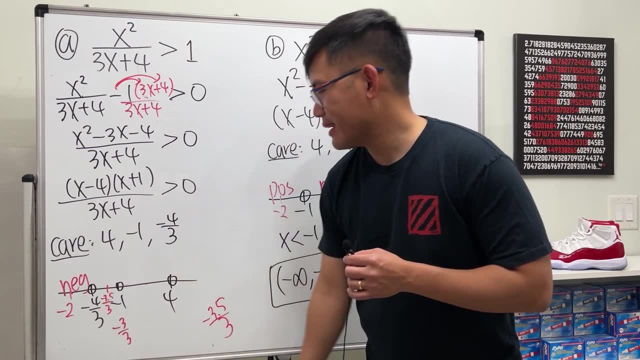 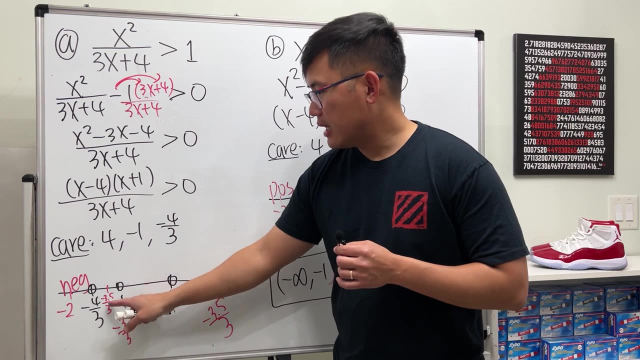 man, let's pick negative 3.5 over 3 for this. Negative 3.5.. Negative 3.5 over 3.. Yeah, All right. When you put this on the bottom we get positive. Negative put here is negative. 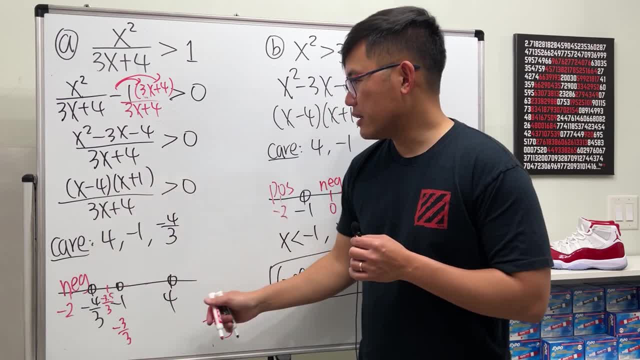 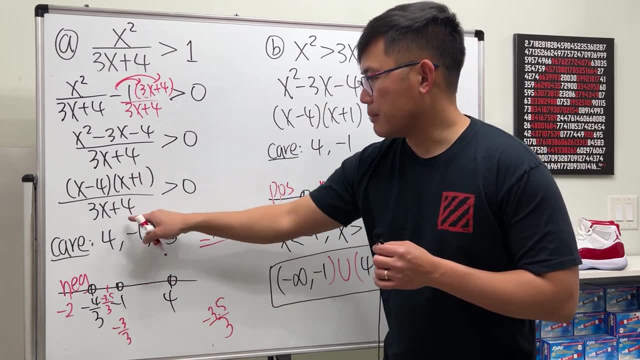 This is less than negative 1, so this is negative. So together again, when we put this right here, we get negative. When we put this right here, it's negative. But on the bottom, when we put this right here, the 3 cancel. 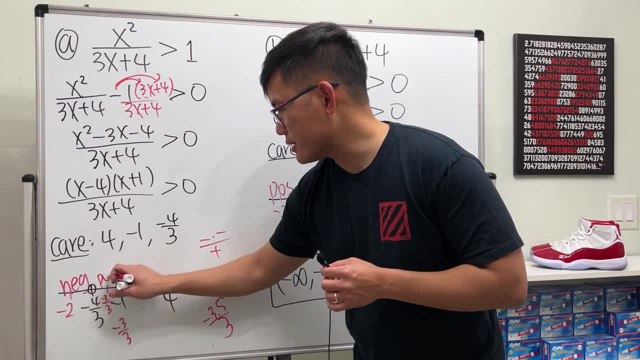 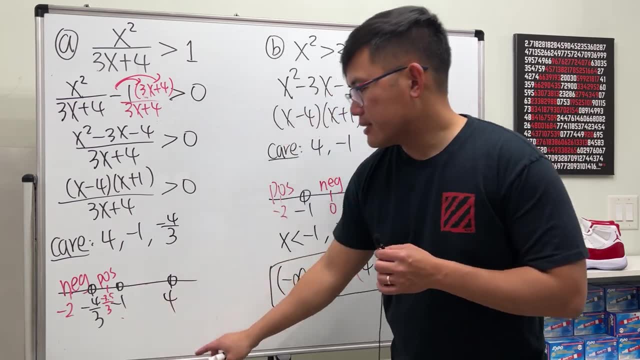 In fact we get positive. So altogether we get positive. I forgot what I said earlier, But the result is positive. for that, Yeah, All right. Next, pick a number from negative, between negative 1 and 4.. Let's say 0.. 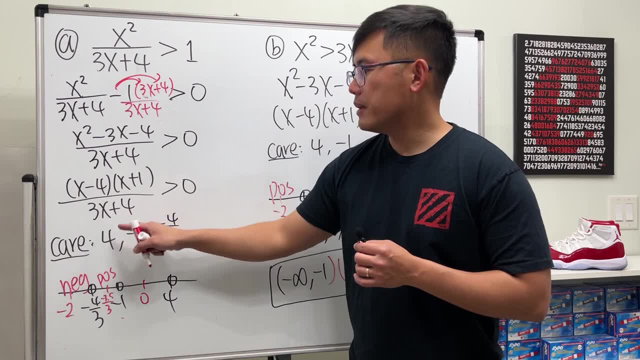 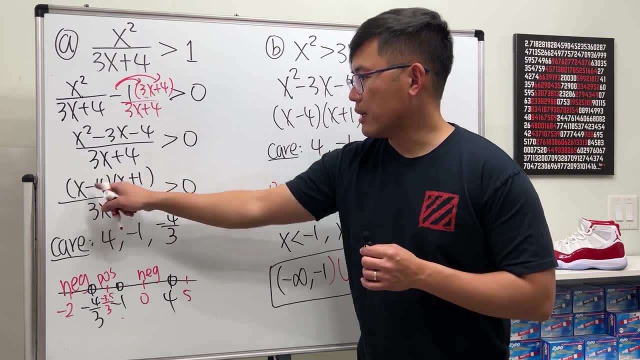 Put it here as negative, Put it here as positive, Put it here as positive, So altogether it's negative. Lastly, pick a number bigger than 4. Let's say 5. Positive, positive, positive, So positive Yeah. 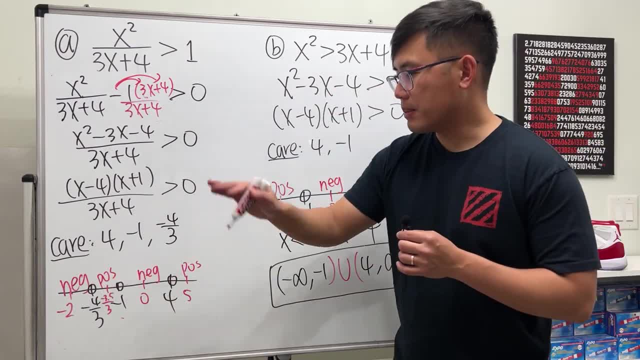 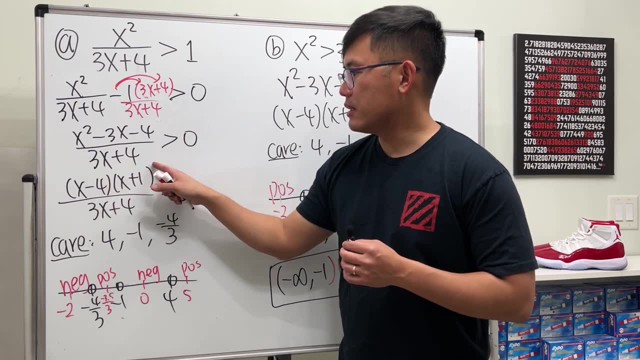 It's good that we don't have signs like positive positive Or negative, negative, that is, the alternates, And the reason for this to happen is because you don't have any like even degrees here, even power. so yeah, 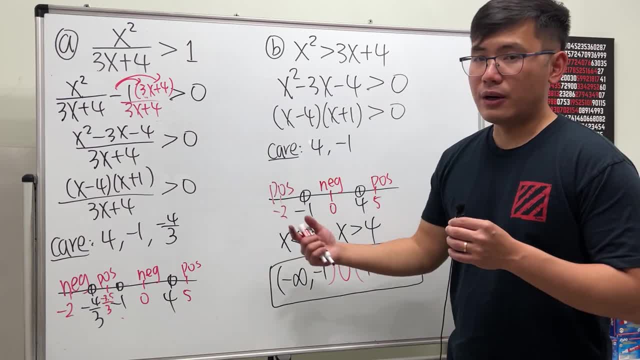 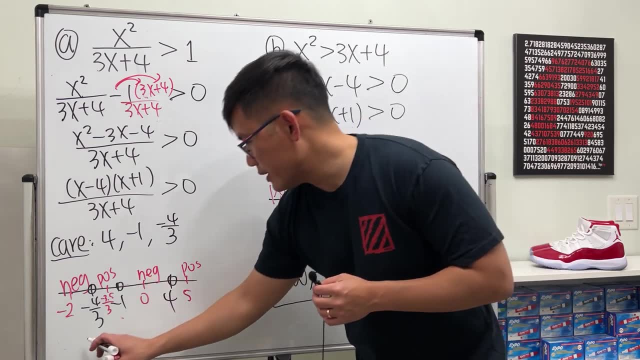 But anyway do. the sign chart is the safest way Now in order for us to get positive. we care about this and that. So the answer, I'll just write this in interval notation: We get negative 4 over 3 to negative 1.. 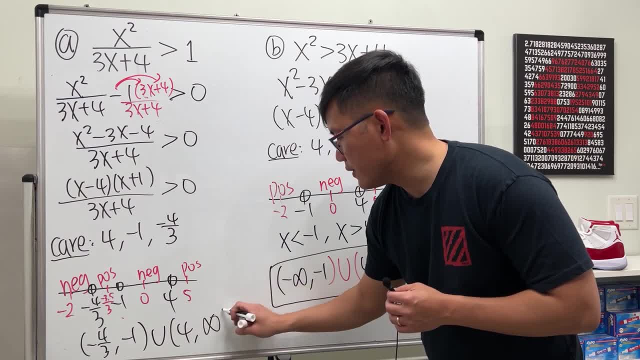 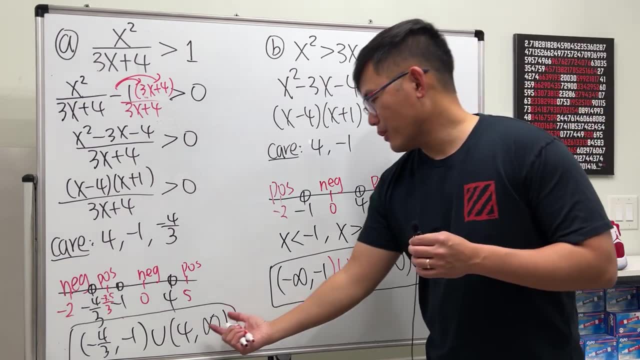 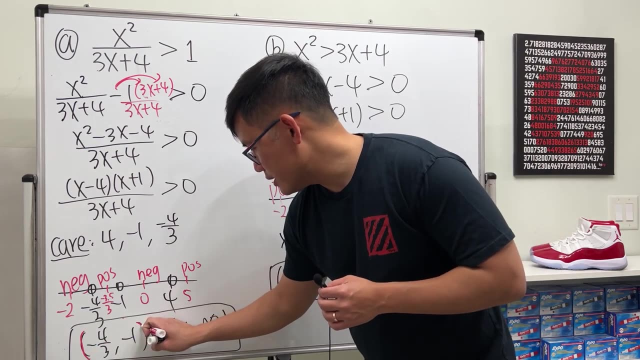 And then union 4 to infinity. So, as you can see, these two things are quite different, although they have one part being the same, though, but the other parts no. And again, these are interval notations. We are not including endpoints right here.